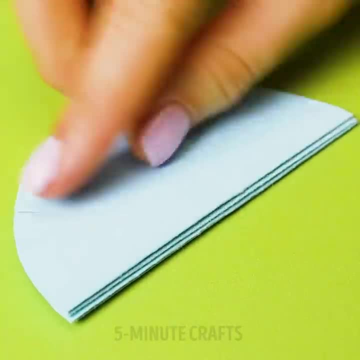 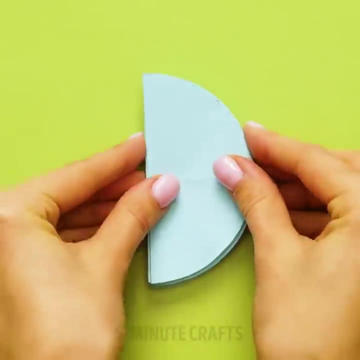 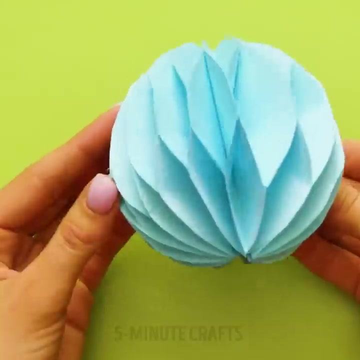 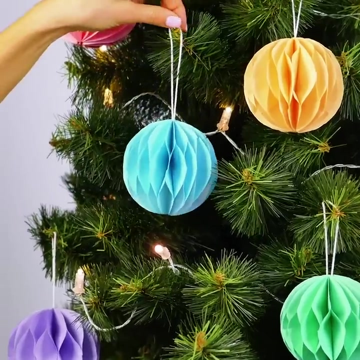 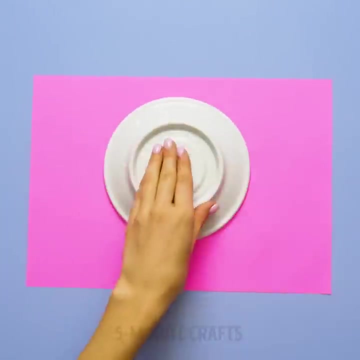 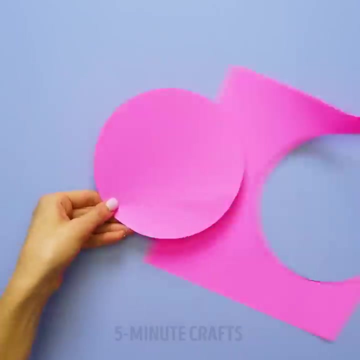 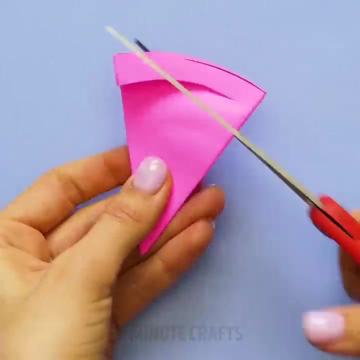 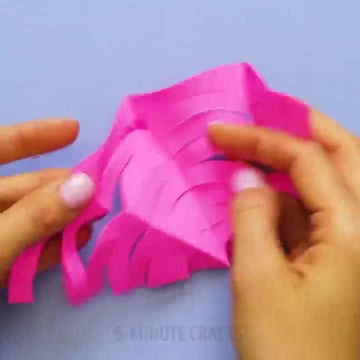 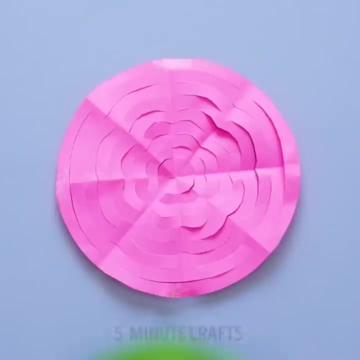 Can you love me again? I need Come on love me the way you did. Am I the one to know you? I just can't change my emotions. Come on, love me again. Oh, oh, oh, oh, oh, oh, oh. 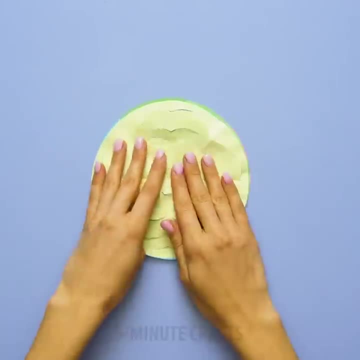 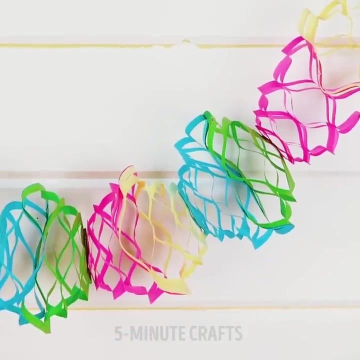 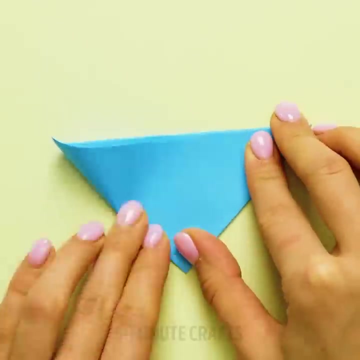 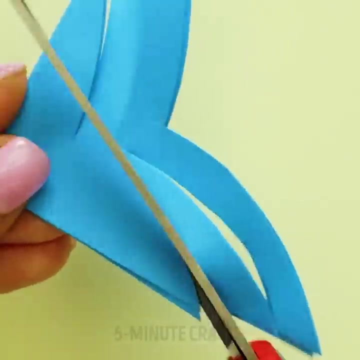 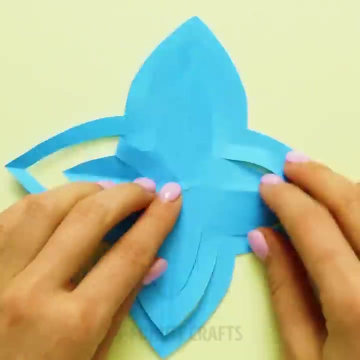 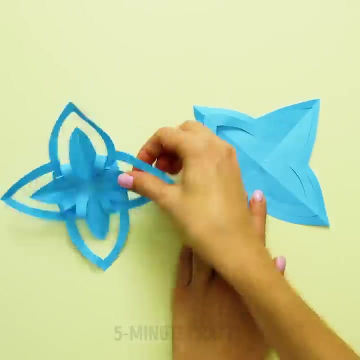 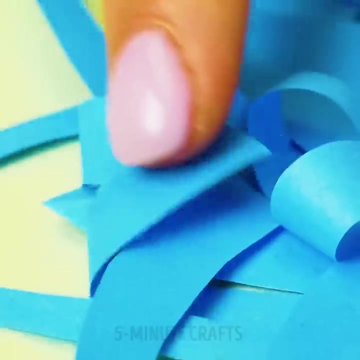 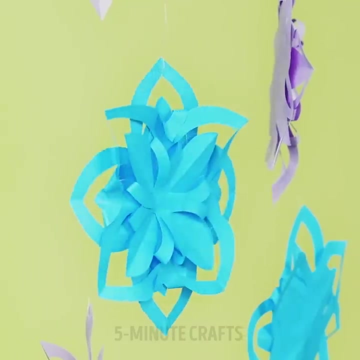 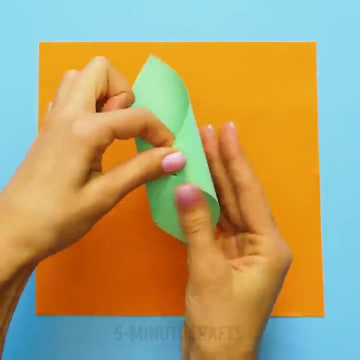 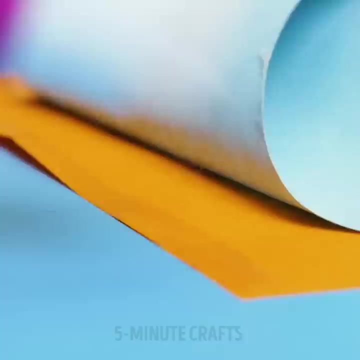 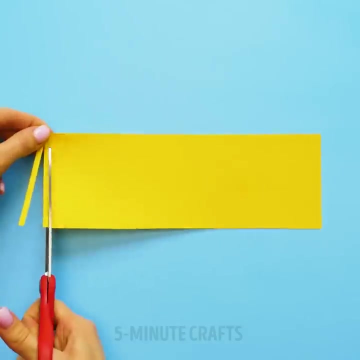 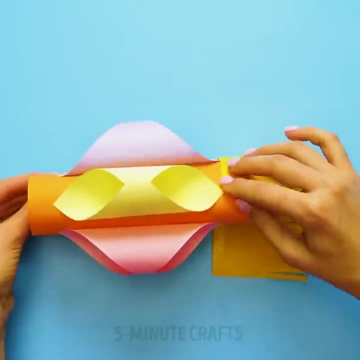 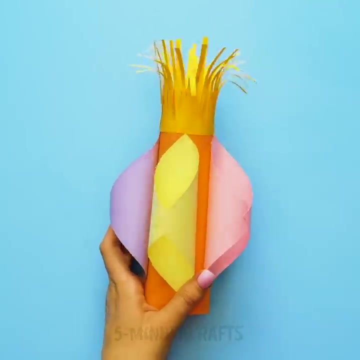 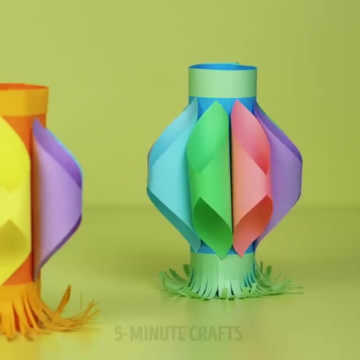 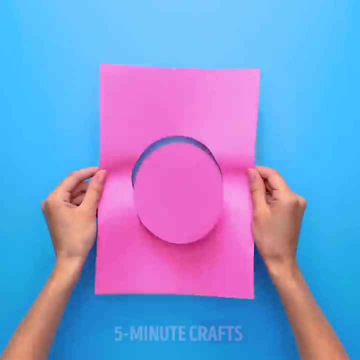 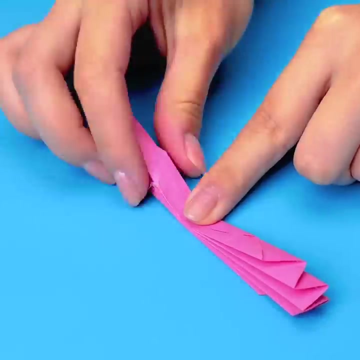 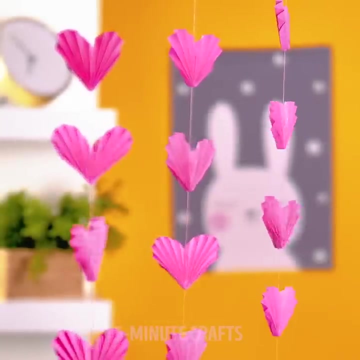 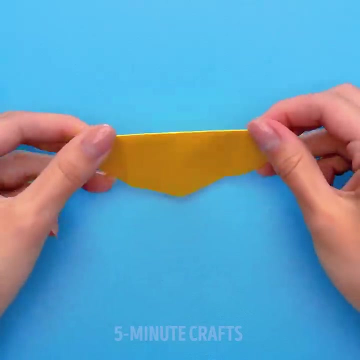 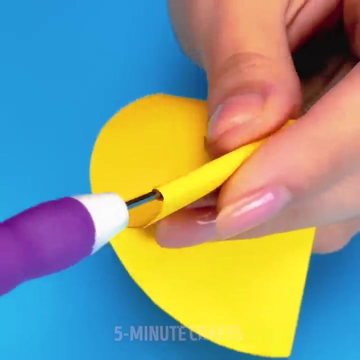 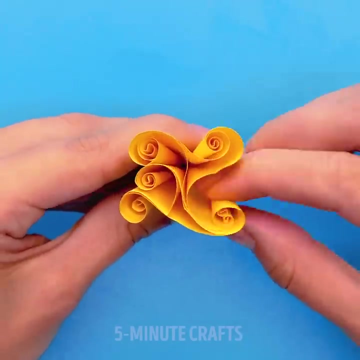 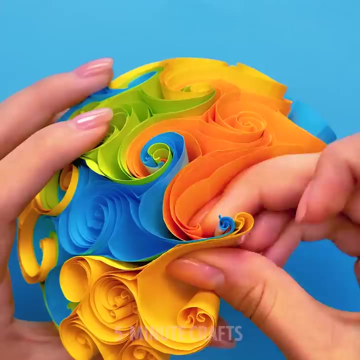 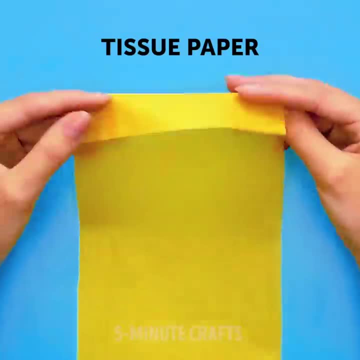 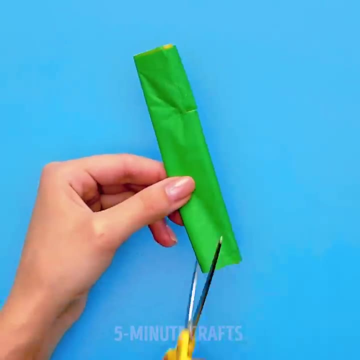 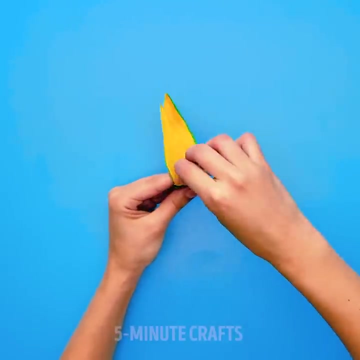 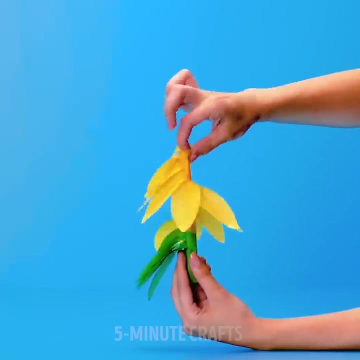 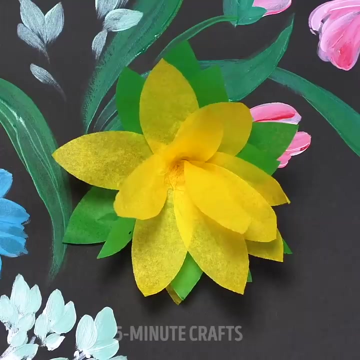 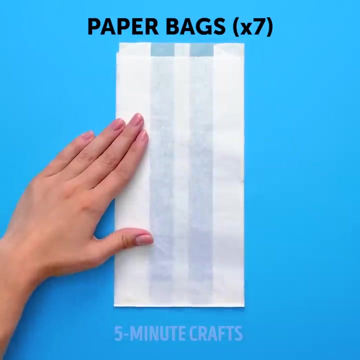 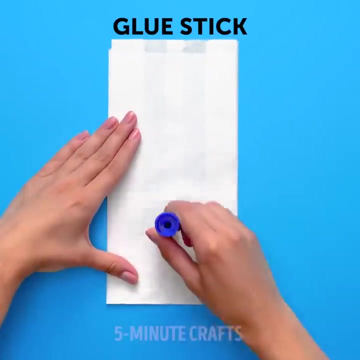 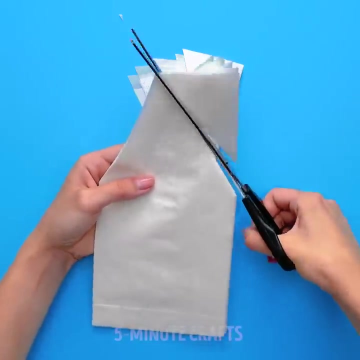 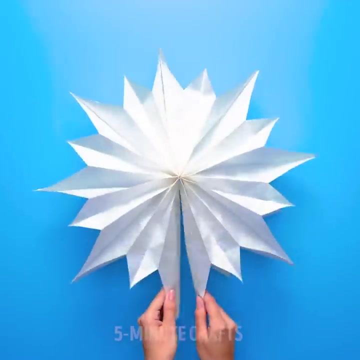 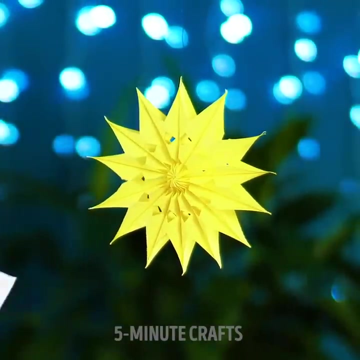 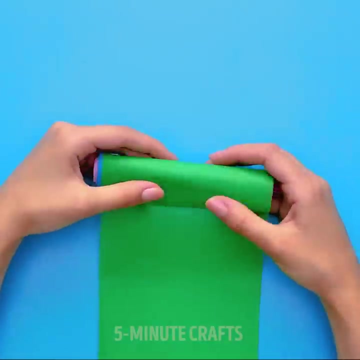 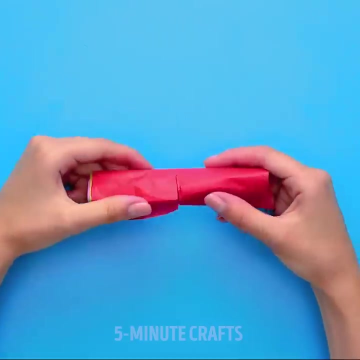 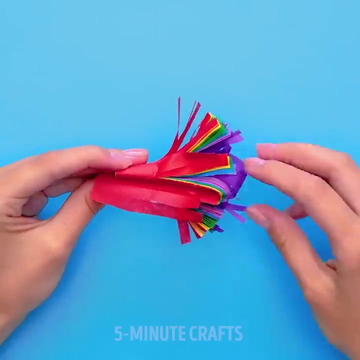 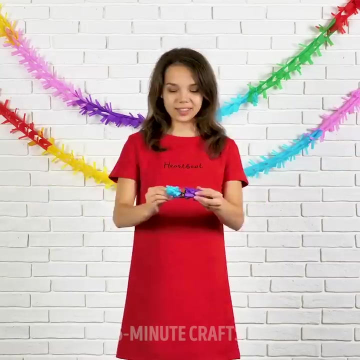 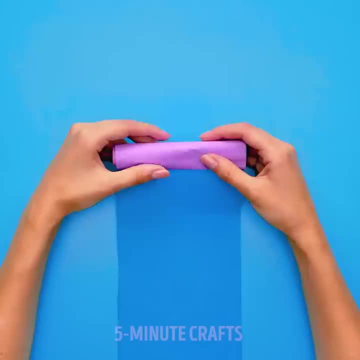 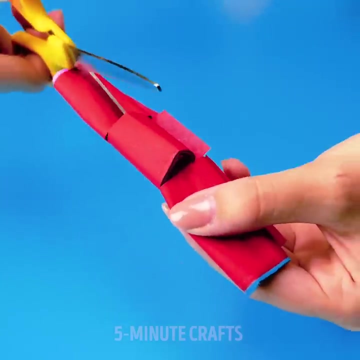 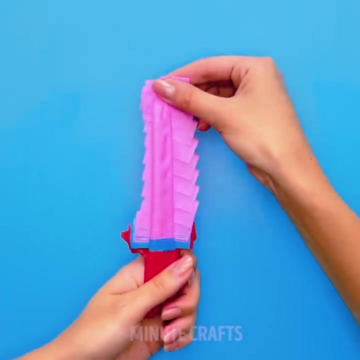 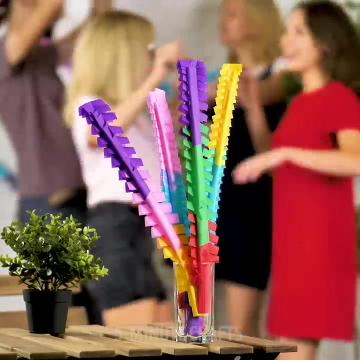 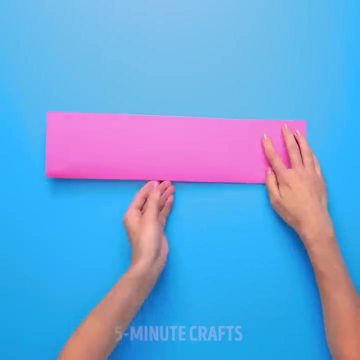 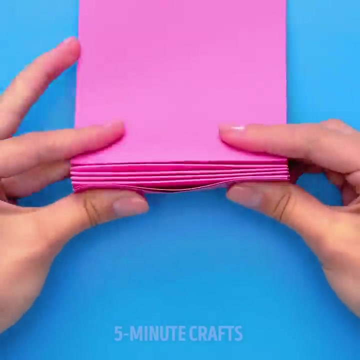 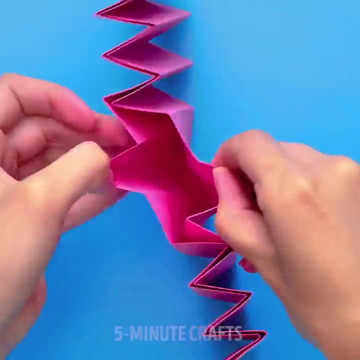 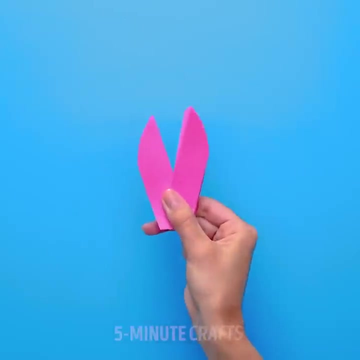 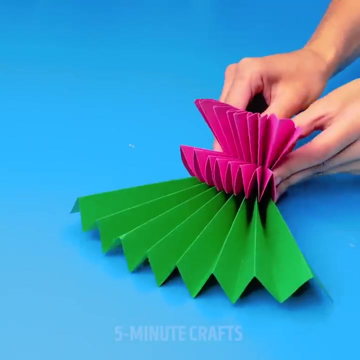 Come on, love me again. You're all I need. Can you love me again? I mean, come on, love me the way you did. I just can't change my emotions. I just can't change my emotions. I just can't change my emotions. But, baby, you're gonna love me again. 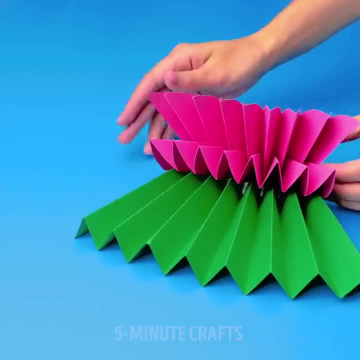 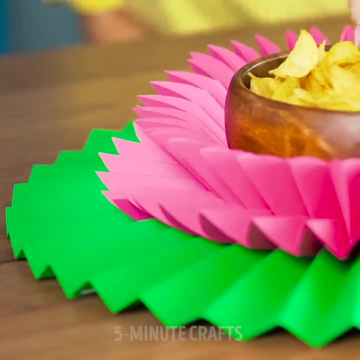 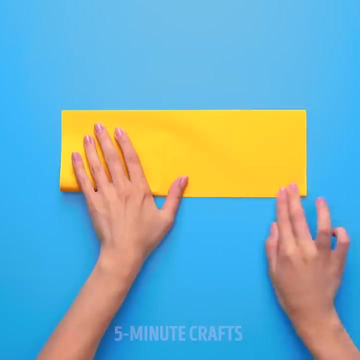 Love me again. Yeah, I paid my dues to show you I'm not the same. It has cost me much, but I will do it again. So, baby, come on, love me again, Love me again. I know I messed it up, but in my soul. I know I messed it up, but in my soul I feel the love for you that's out of control. Sometimes I feel like I can make you whole. I just can't change my emotions. Come on, love me again. You're all I need. Can you love me again? 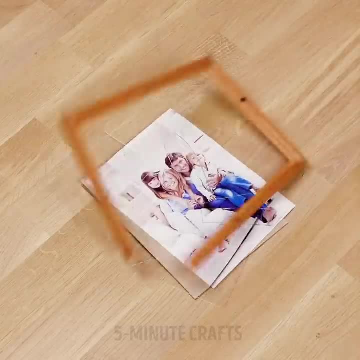 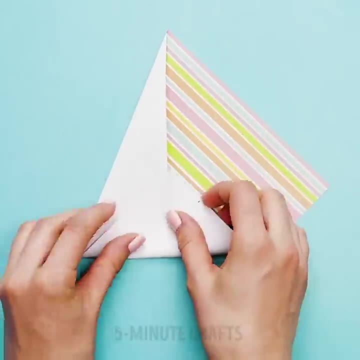 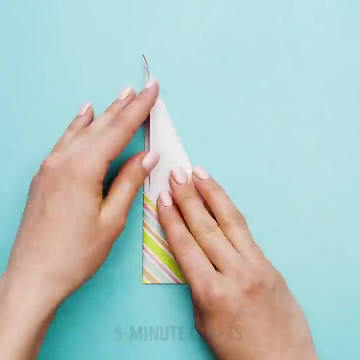 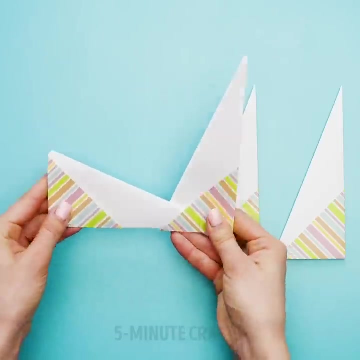 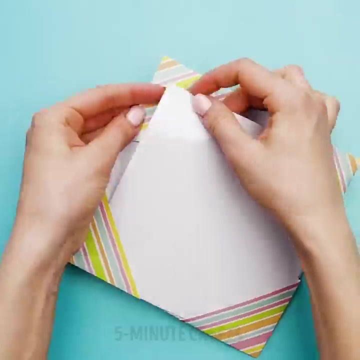 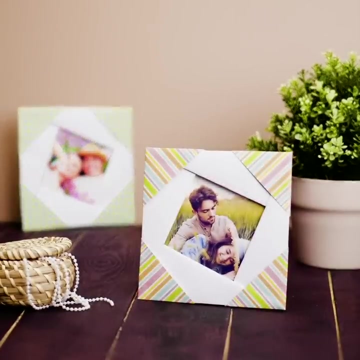 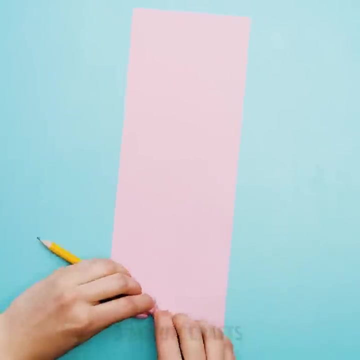 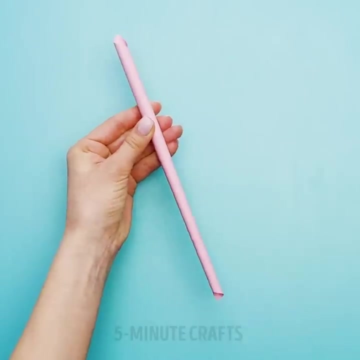 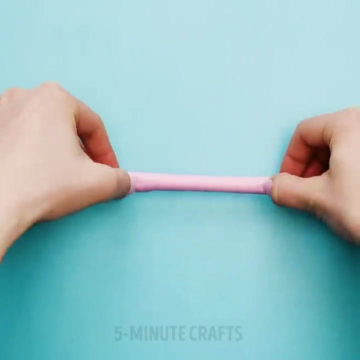 I mean: come on, love me the way you did. I just can't change my emotions. I mean: come on, love me again. You're all I need. But, baby, you're gonna love me again, Love me again. I know I messed it up, but in my soul I feel the love for you that's out of control. Sometimes I feel like I can make you whole. I just can't change my emotions. No, no, I can't beat anything I wanna hold. So we'll get everything to say that it's true, Not if your look or love me or you. 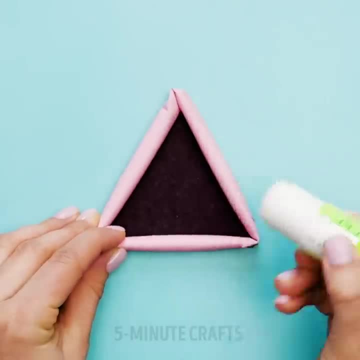 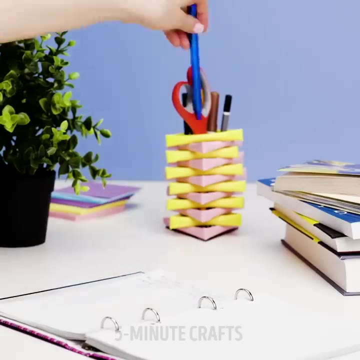 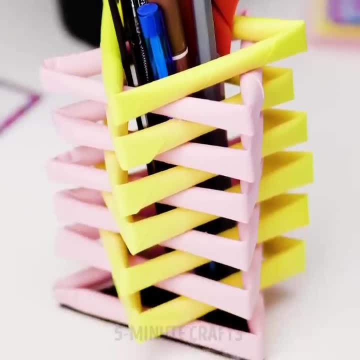 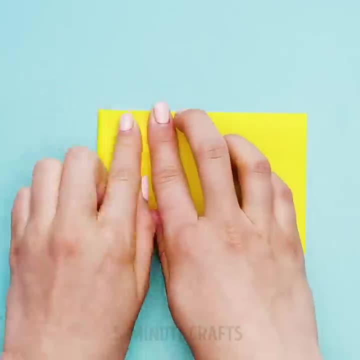 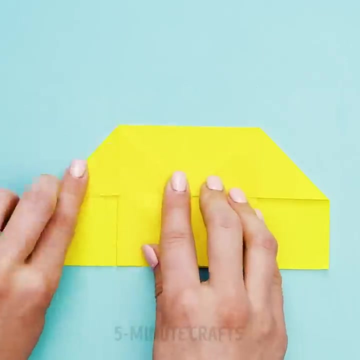 I'm still in love with you. it's out of control. Sometimes I feel like I can make you whole. I just can't change my emotions. There isn't anything I wouldn't do To prove that everything I say is true. And if you love me, I can love in you. 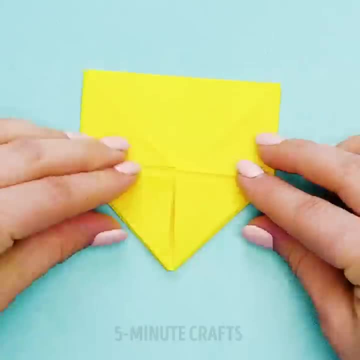 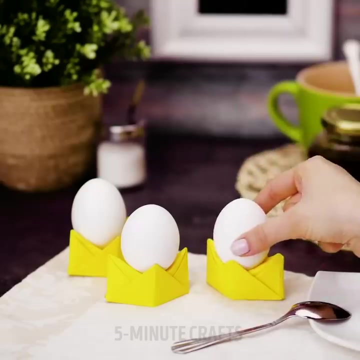 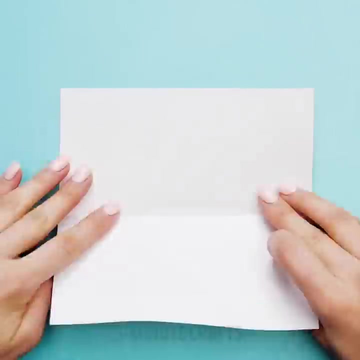 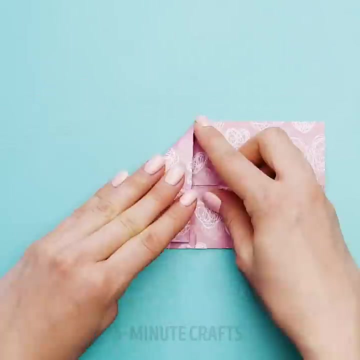 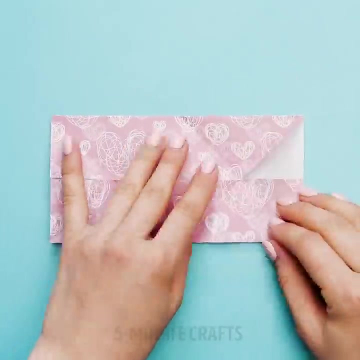 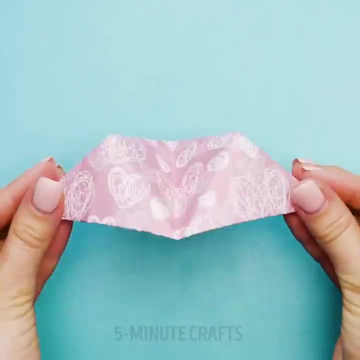 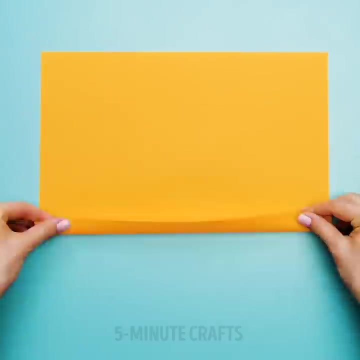 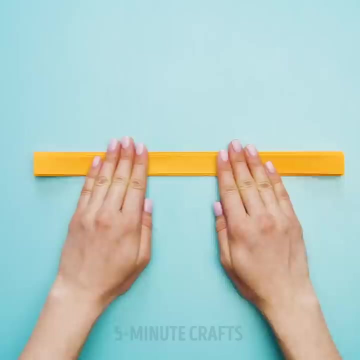 I just can't change my emotions. Come on, love me again. You're all I need. can you love me again? I need someone to love me the way you did. I just can't change my emotions. Maybe I know it's my time to save. 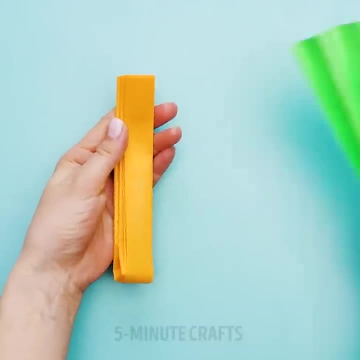 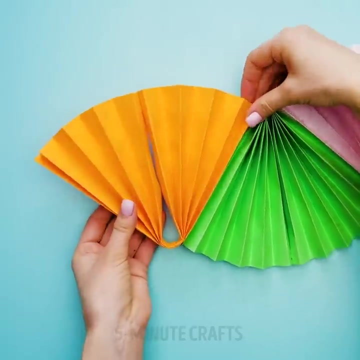 But, baby, I know it's my time to save, But, baby, I know it's my time to save. You're gonna love me again. love me again. Yeah, I paid my dues to show you I'm not the same. It has cost me much, but I will do it again. 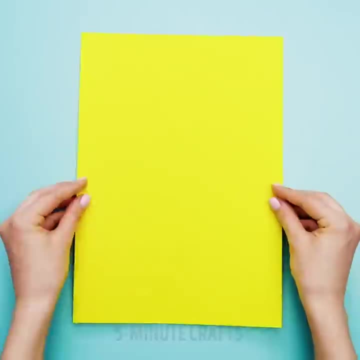 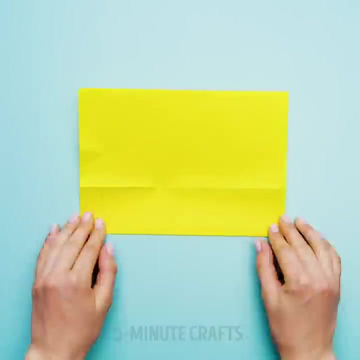 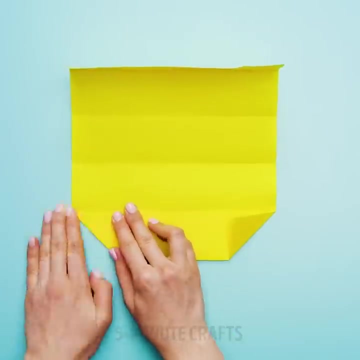 So, baby, I'm gonna love you again, love you again. I don't wanna see a book in my soul. I feel the love for you. it's out of control. Sometimes I feel like I can make you whole. I just can't change my emotions. 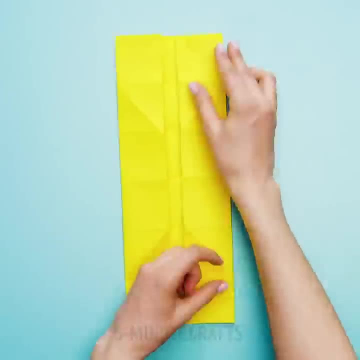 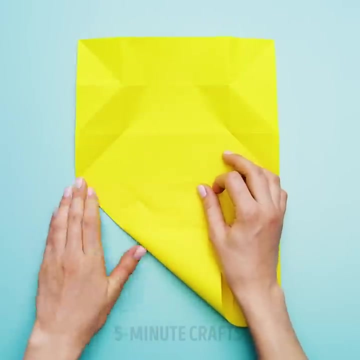 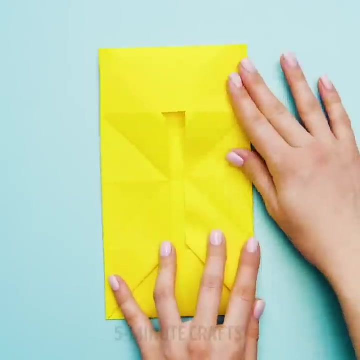 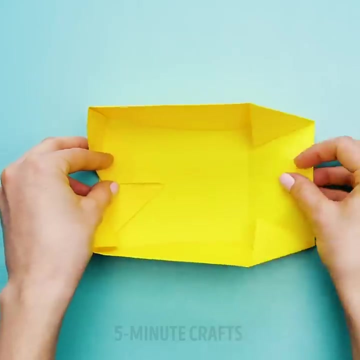 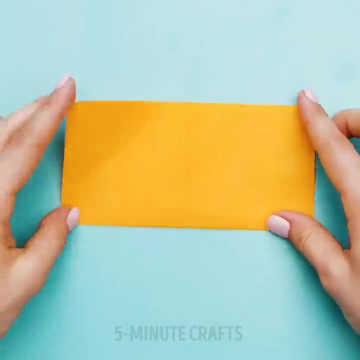 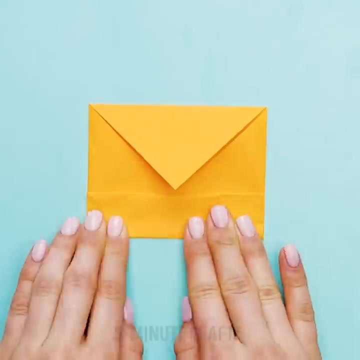 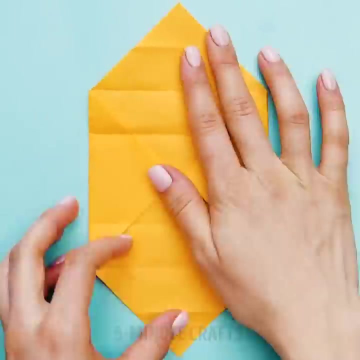 Come on, let me in. you're all I need. Can you let me in? I need, I need. Come on, let me do it, do it, do it. I just can't change my emotions. I don't wanna see a book in my soul. I feel the love for you. it's out of control. Come on, let me in, you're all I need. Can you let me in? I need, I need. Come on, let me in, you're all I need. Can you let me in? I need, I need. 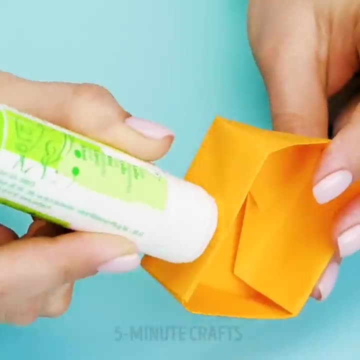 I don't wanna see a book in my soul. I feel the love for you. it's out of control. Sometimes I feel like I can make you whole. I just can't change my emotions. Can you let me in? you're all I need. Can you let me in? you're all I need. 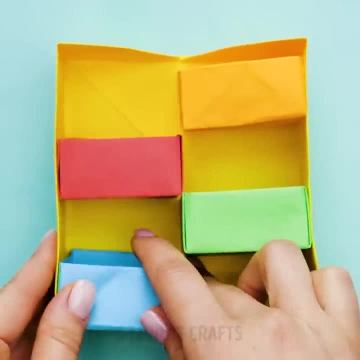 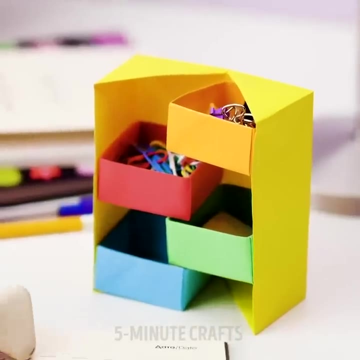 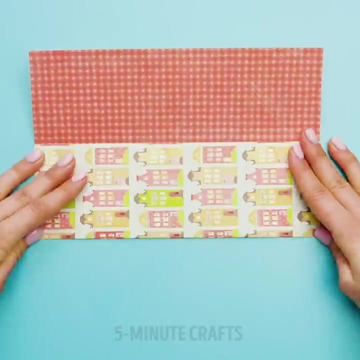 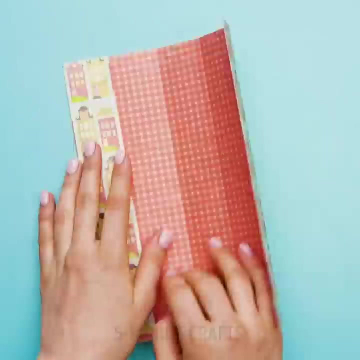 Can you let me in? you're all I need. So, through this, everything, this thing is true. Everything I think of is loving you. I just can't change my emotions. I know I lost it, but look at my soul. I still love for you. it's out of control. 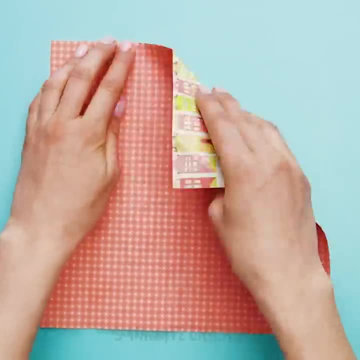 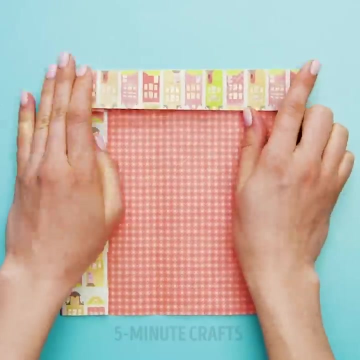 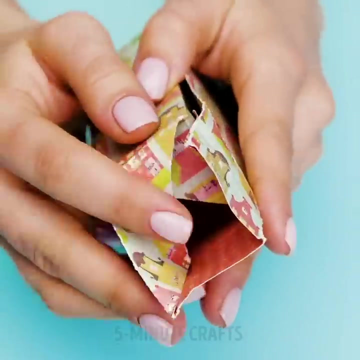 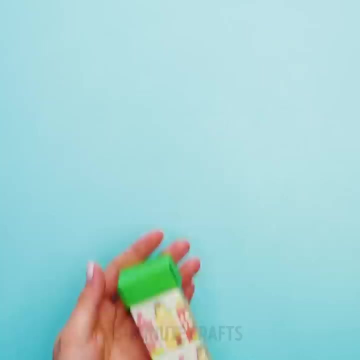 Sometimes I feel like I can make you whole. I just can't change my emotions. There isn't anything I wouldn't do To prove that everything I say is true And if you love me, I can love in you. I just can't change my emotions. Come on, love me again. 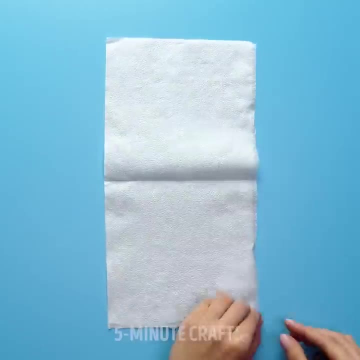 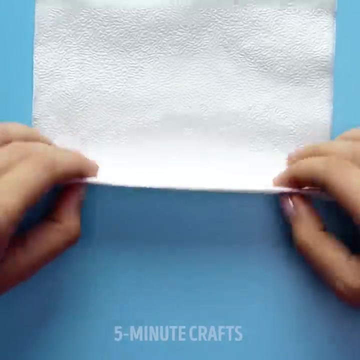 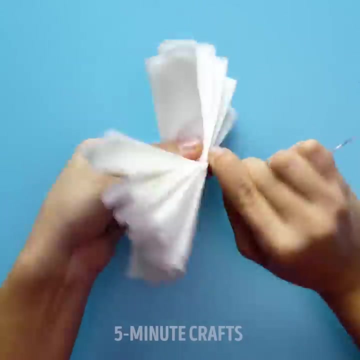 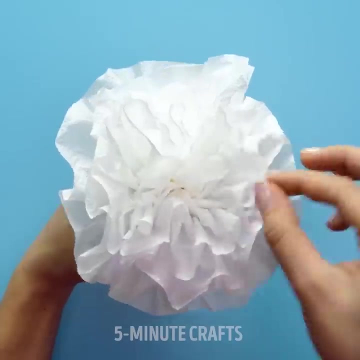 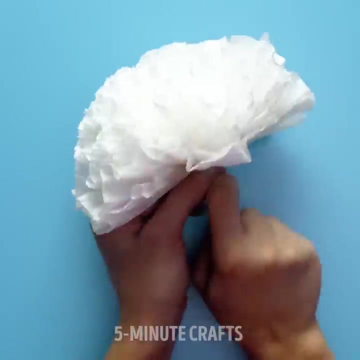 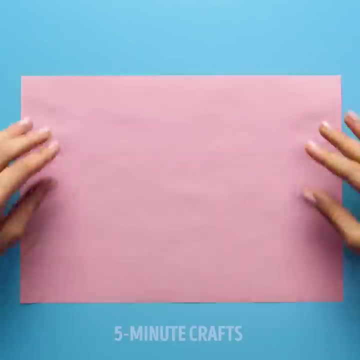 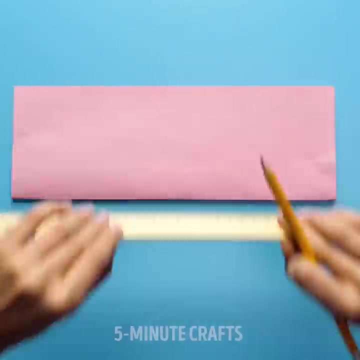 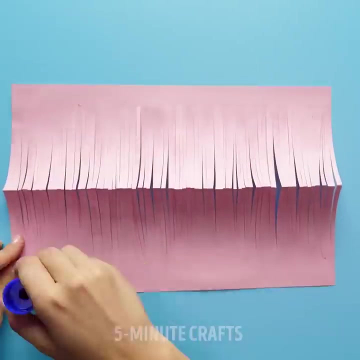 You are a leaf. can you love me again? A leaf? come on, love me. come on, love me. I just can't change my emotions, Baby. I know this might sound insane, But baby, you're gonna love me again. Come on, love me again. 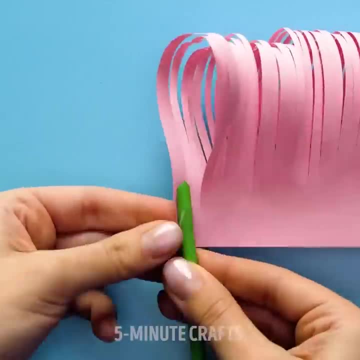 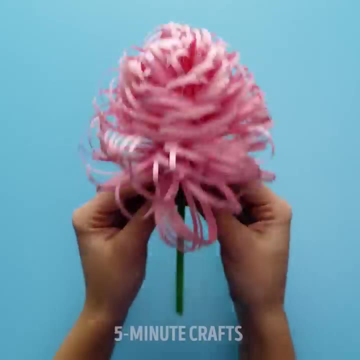 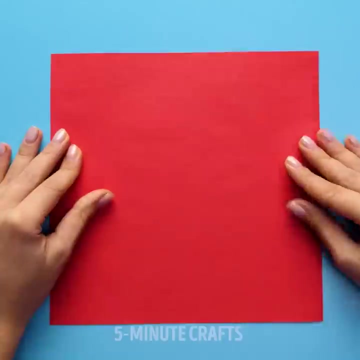 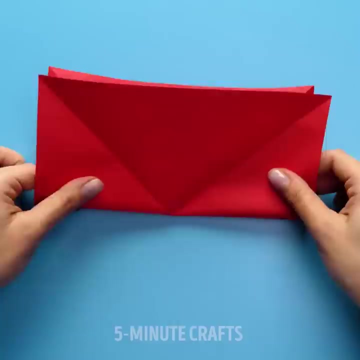 Love me again. Yeah, I paid my dues to show you I'm the same. It cost me much, but I would do it again. So, baby, come on, love me again, Love me again. I know I lost it, but look at my soul. I still love for you. it's out of control. 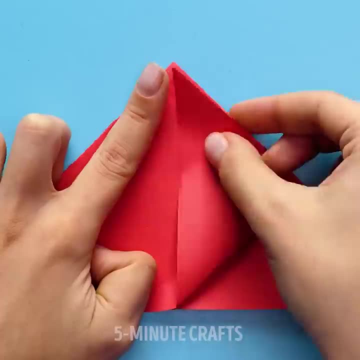 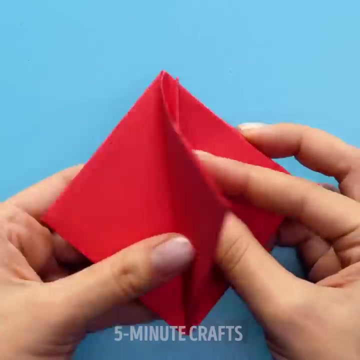 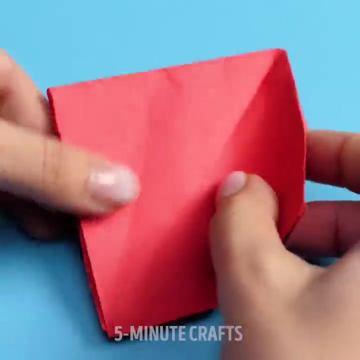 Sometimes I feel like I can make you whole. I just can't change my emotions. Come on, love me again. You are a leaf. can you love me again, A leaf? come on, love me. come on, love me again. I just can't change my emotions. 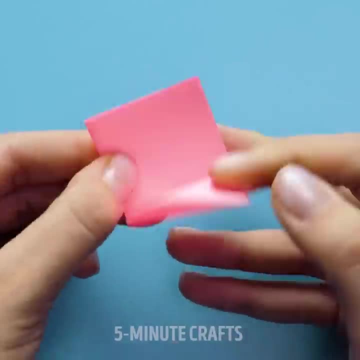 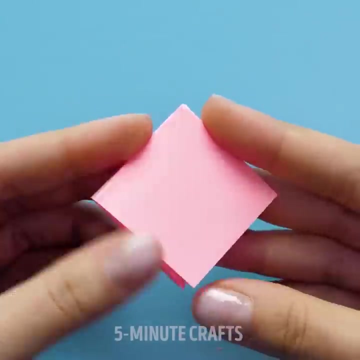 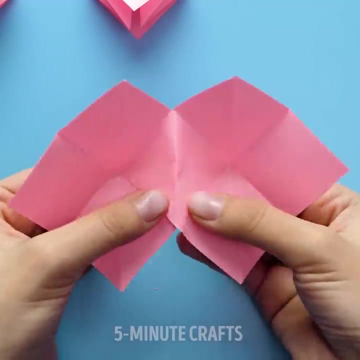 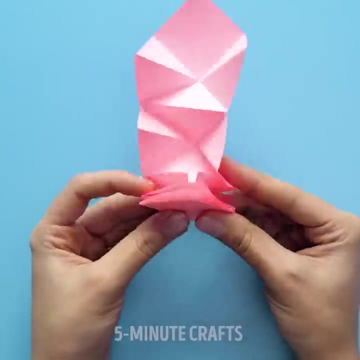 Baby, I know this might sound insane, But, baby, you're gonna love me again. I just can't change my emotions, Baby. I know I lost it, but look at my soul. I still love for you. it's out of control. Sometimes I feel like I can make you whole. 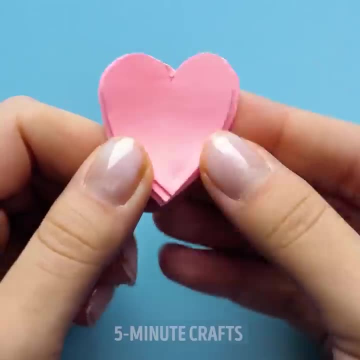 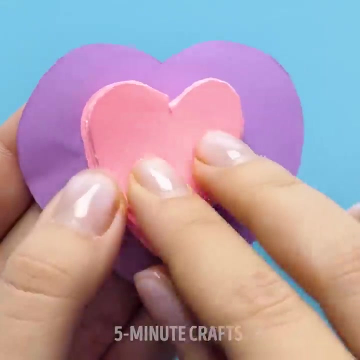 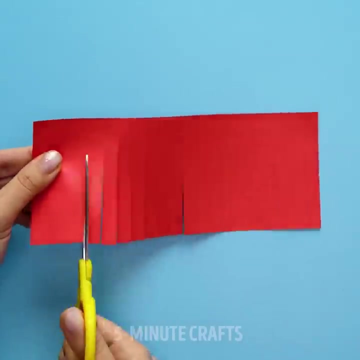 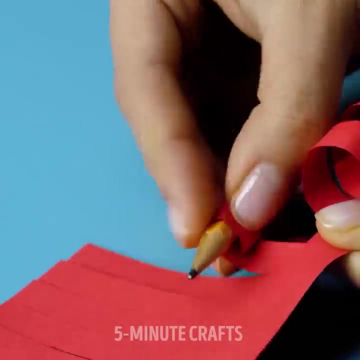 But I can make you whole, I just can't change my emotions, Baby. anything I would do To prove that everything I say is true. And if you look me up, you love me, you. I just can't change my emotions. I know I lost it, but look at my soul. 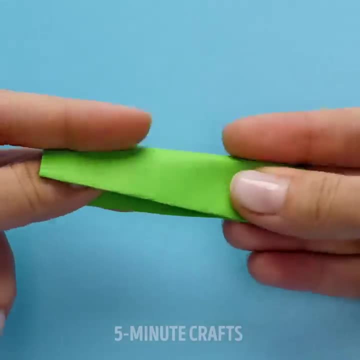 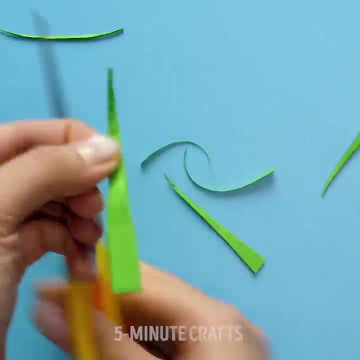 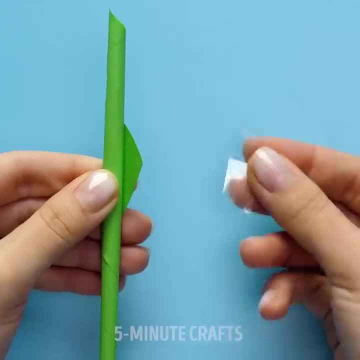 I still love for you. it's out of control. I feel it for you. it's out of control. Sometimes I feel like I can make you whole. I just can't change my emotions. There isn't anything I wouldn't do To prove that everything I say is true. 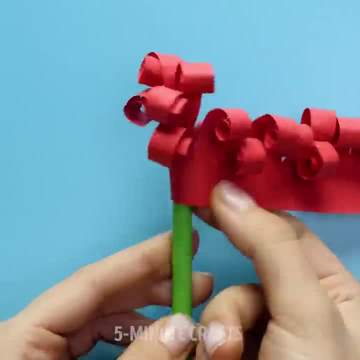 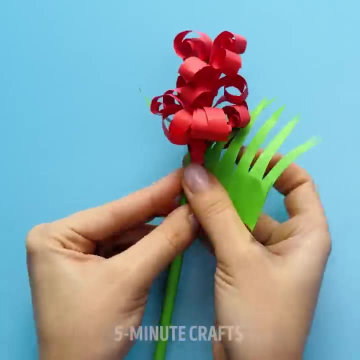 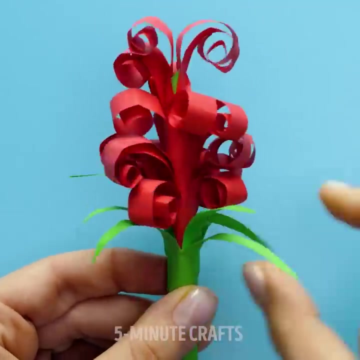 And if you look me up, you love me. you, I just can't change my emotions. Come on, love me again, You're all I need. can you love me again? I mean, come on, love me the way you did. I just can't change my emotions. 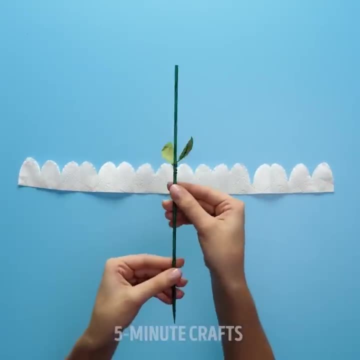 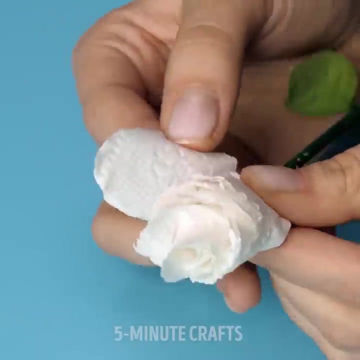 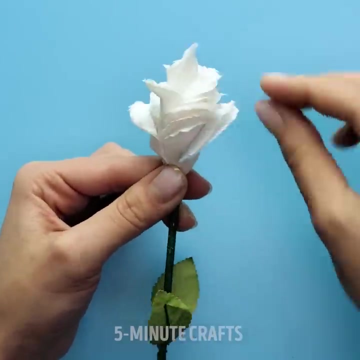 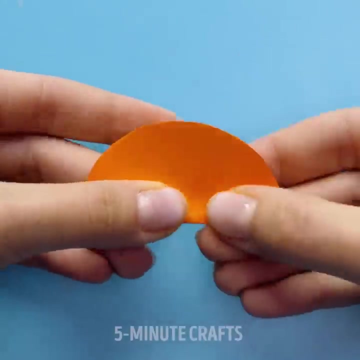 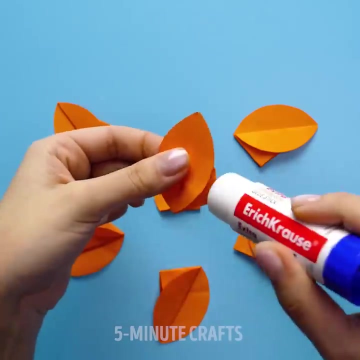 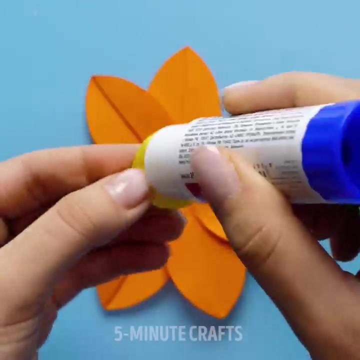 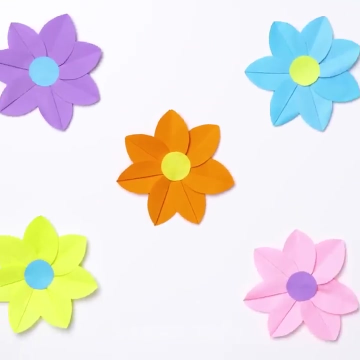 I just can't change my emotions. I mean, my dues are sure you are not the same. It has cost me much, but I would do anything. So, baby, come on, love me again, Love me again. I know I messed it up in my soul. 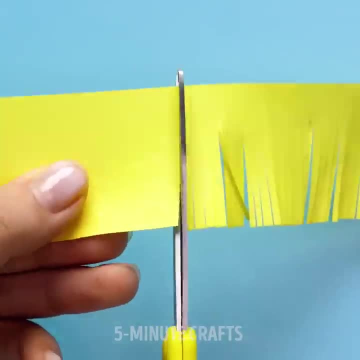 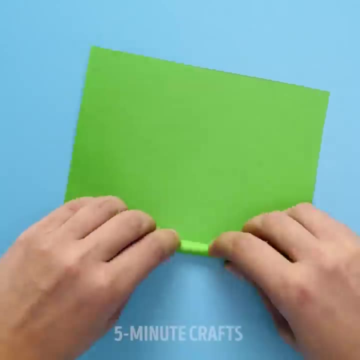 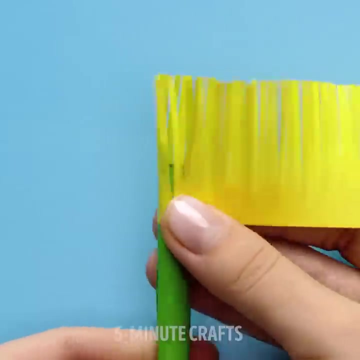 I feel love for you that's out of control. Sometimes I feel like I can make you whole. I just can't change my emotions. I mean, come on, love me again. Oh, come on, love me again. You're all I need. can you love me again? 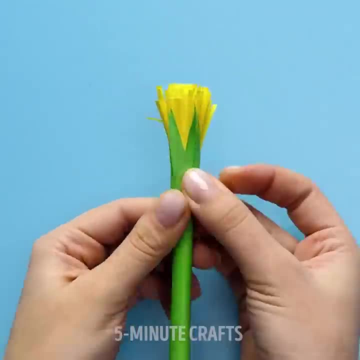 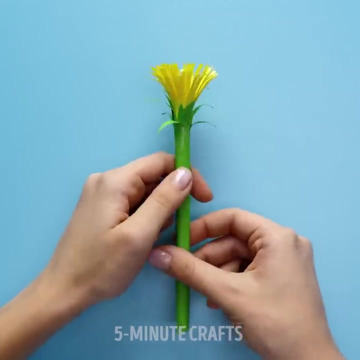 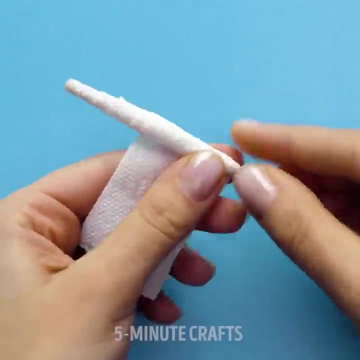 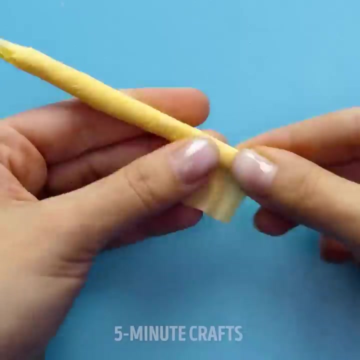 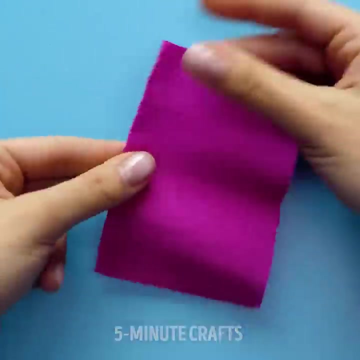 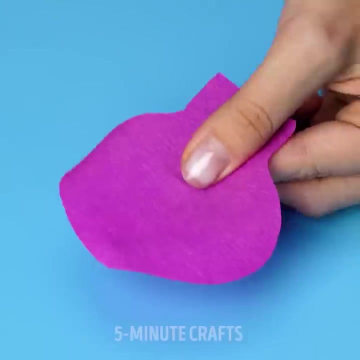 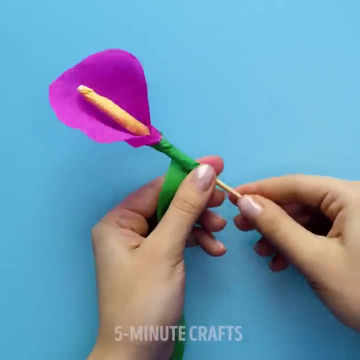 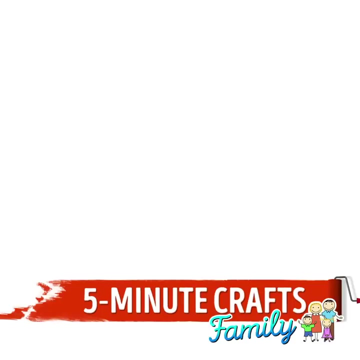 I mean, come on, love me the way you did. I just can't change my emotions. I know I messed it up in my soul. I feel love for you that's out of control. Sometimes I feel like I can make you whole. I just can't change my emotions.